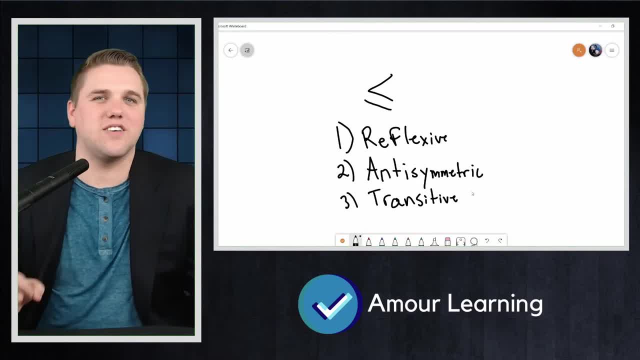 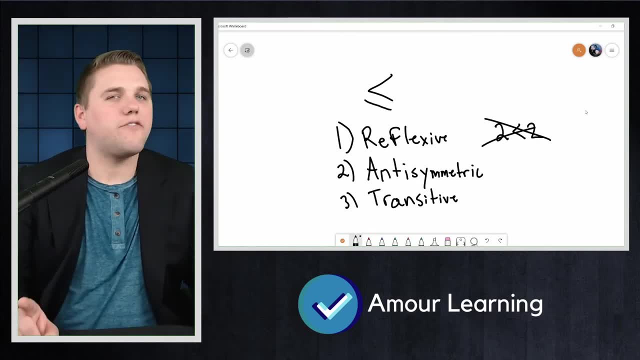 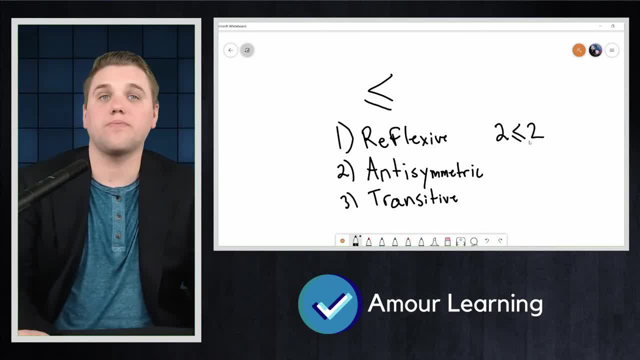 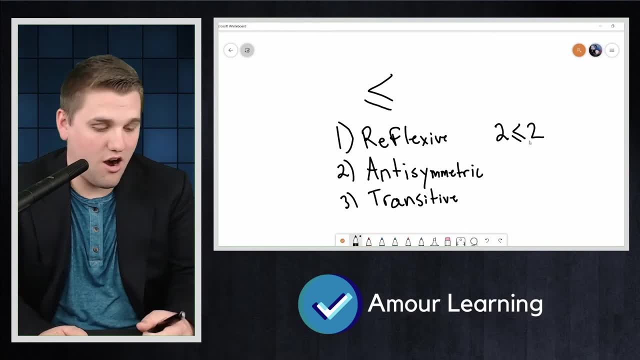 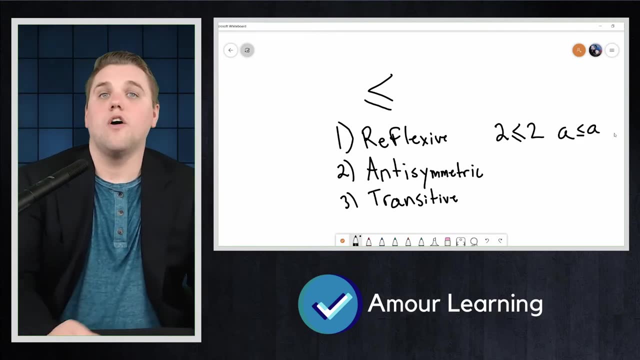 Let's look at the less than or equal to symbol, And so, in fact, this is true for any a in the real numbers, or integers, or whichever you want to use. In general, this is true for all real numbers, again integers, whichever universe you'd like to work with. What about the anti-symmetric property? 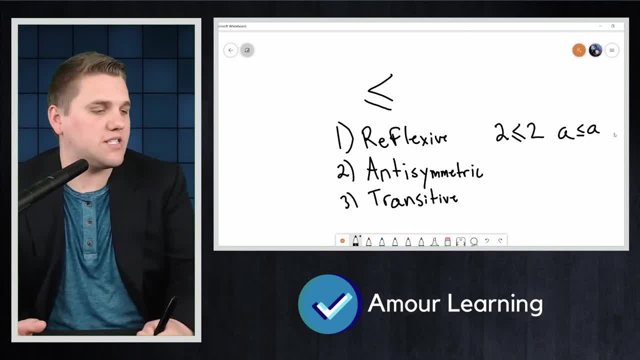 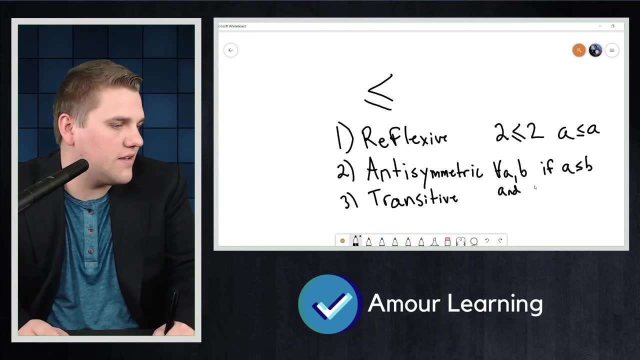 What does that mean? Well, what this means is that for all elements in our universe, for all a and b, that if a is less than or equal to b and b is less than or equal to a, then that just means a and b. 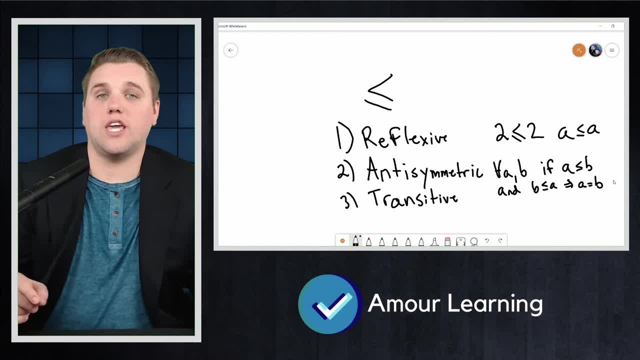 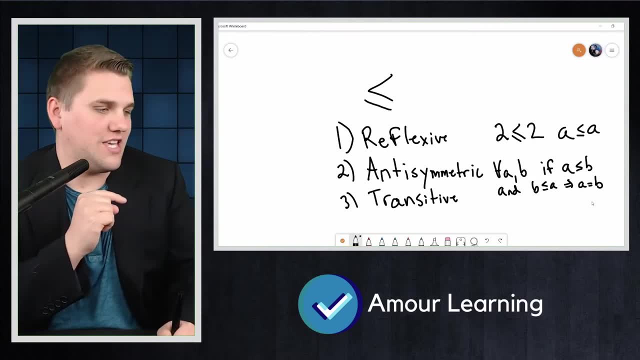 are equal to each other. Now, this can be tricky sometimes because in the definition of partial orderings here there is a use of the equal symbol. So if a is less than or equal to b, then it's a different symbol, which is an equivalence relation. It's a different relation. 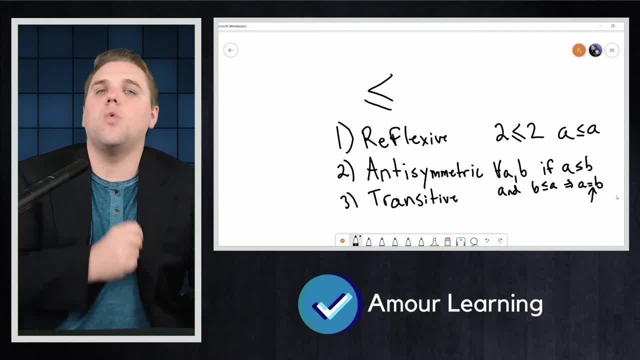 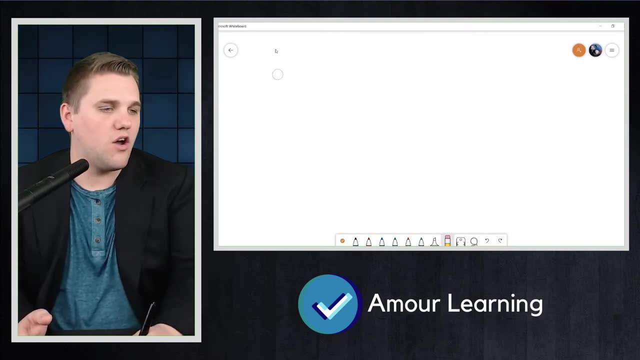 When we say a equals b- in this context, though, we just mean that a and b are literally the same element in the universe. Let's take a look at an interesting partial ordering of the natural numbers. So I'm actually going to write here- I'm going to clear this off our universe- that 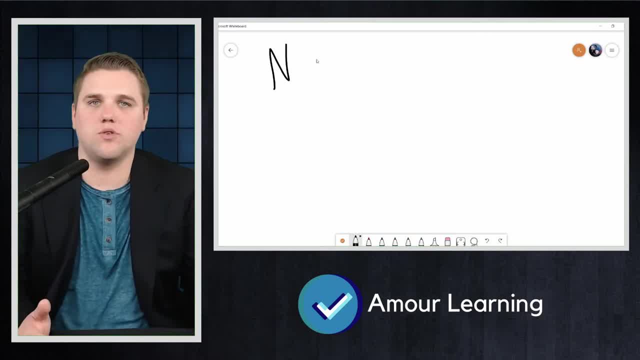 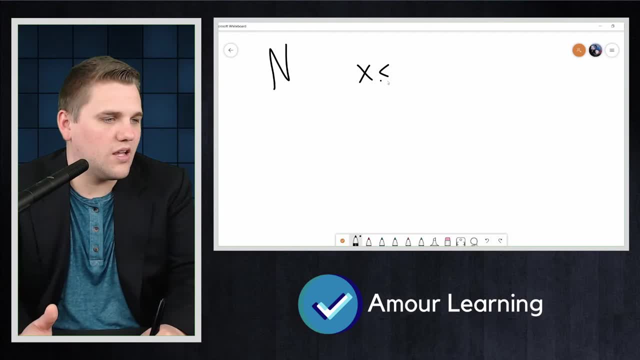 we're working in is n the natural numbers 0,, 1,, 2,, 3, and so on. So we might say that x is less than or equal to, and I'll put quotes here around that- to say: 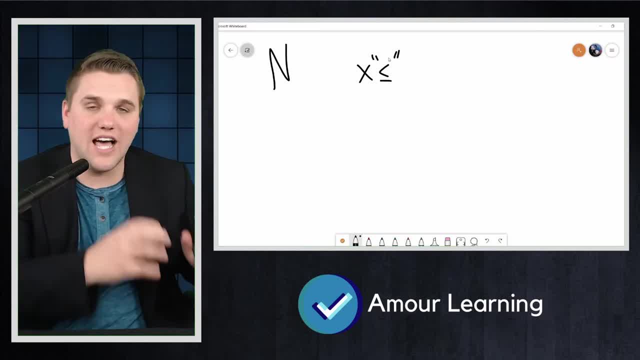 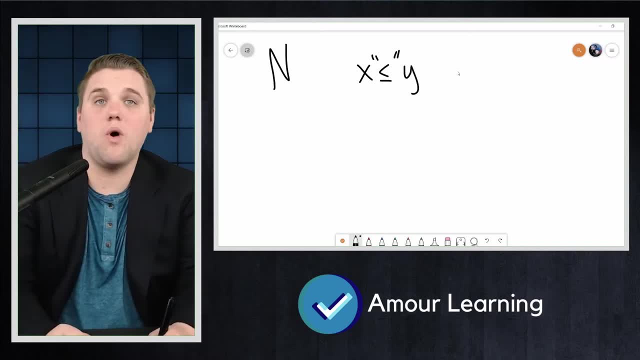 this is not necessarily the same thing as less than or equals. This is just a partial ordering. We might say that x is less than or equal to y or smaller than y if x divides y And we put a vertical line to suggest to say that x divides y. 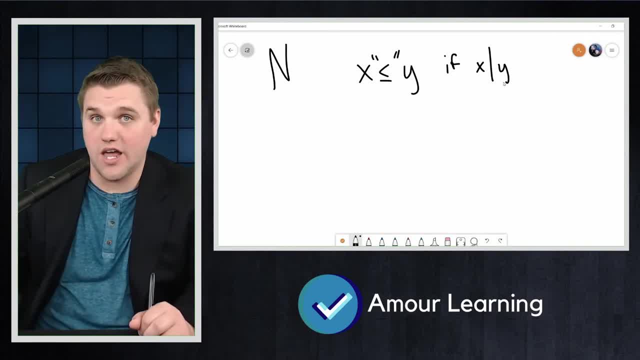 So like: 2 divides 10,, 5 divides 10, 1 divides 10,, 10 divides 10,, 7 does not divide 10, because 7 is not a factor of 10.. This is a partial ordering. This is a partial ordering. 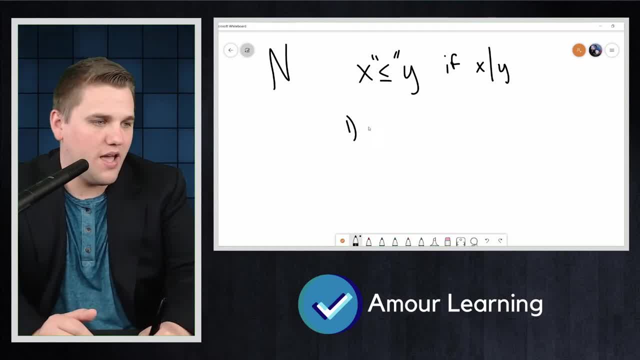 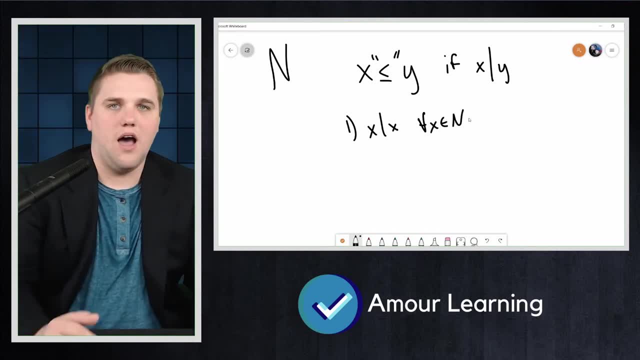 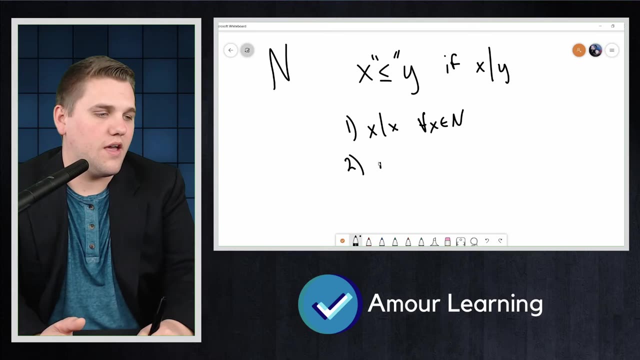 because technically, for the reflexive property, x divides x, for all x in my natural numbers, Every number divides itself. That's definitely true. And then for the second property, if x divides y and y divides x, then x and y are the same. 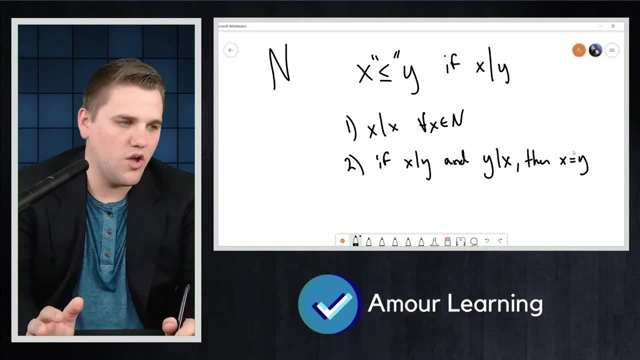 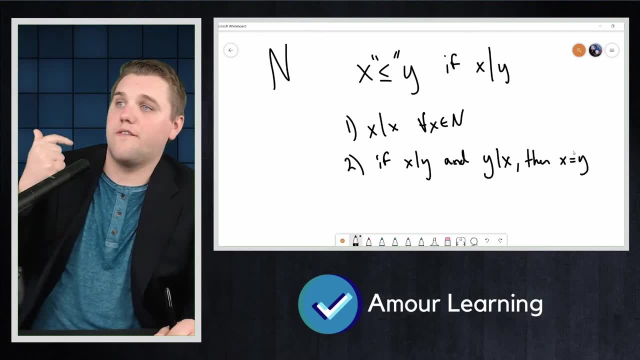 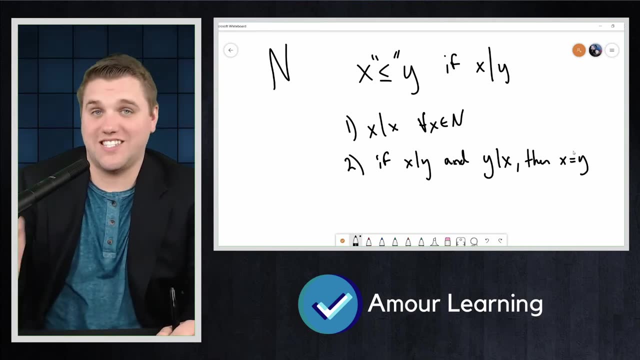 numbers. They're the same natural numbers. This is definitely true. So think of all the elements, for example, that divide 10.. There's 1,, 2,, 5, and 10.. Of those, which of those numbers does 10 divide? Well, 10 doesn't divide 1,. 10 doesn't divide 2,. 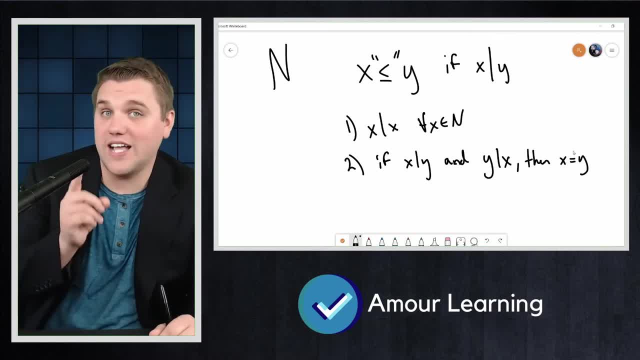 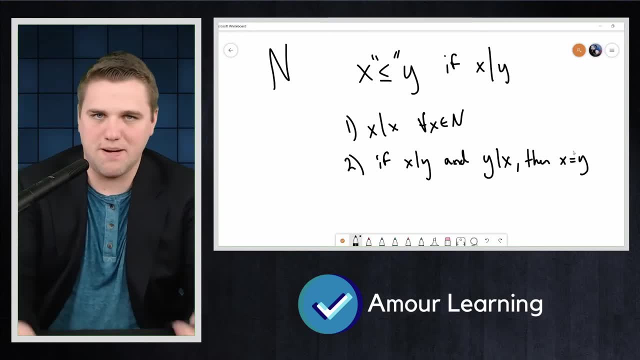 10 doesn't divide 5, but 10 does divide 10.. And so 10 divides 10, and the other direction: 10 divides 10, that means 10 and 10 are the same numbers. That's the second property. 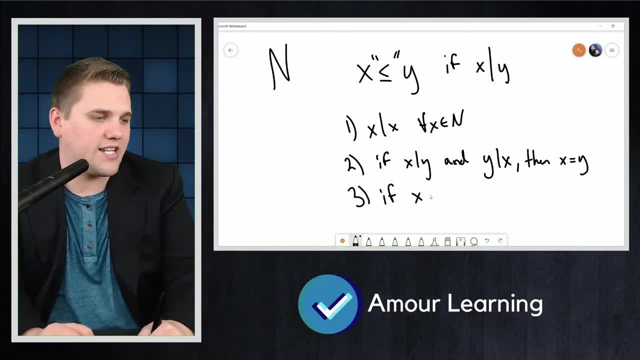 The third property is the transitive property. If x is a factor of y or x divides y and y is a factor of y, then x divides y. And so if x divides y and y is a factor of y, then x divides y. 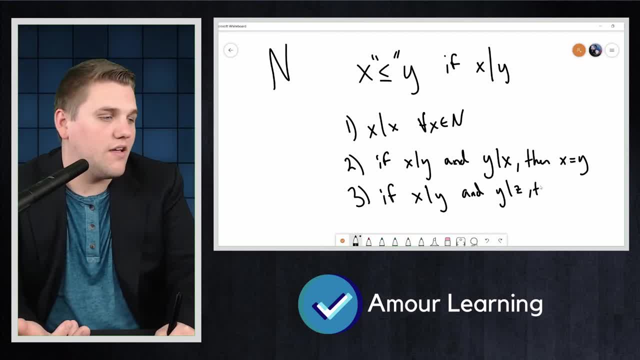 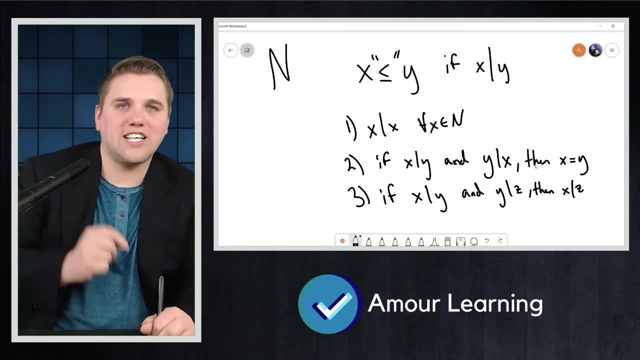 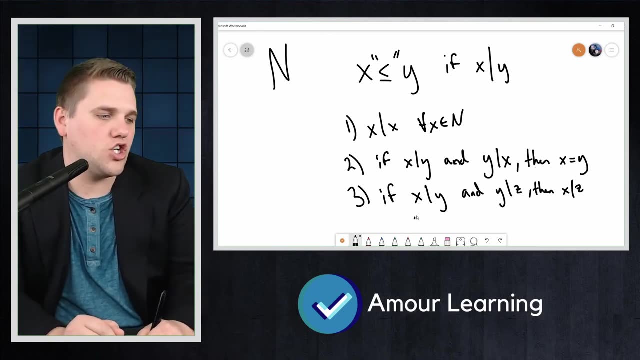 And so if x is a factor of z, which means y divides z, then x divides z. So again, if x is a factor of y, y is a factor of z, then x divides z. We could see this if we say: 2 divides 10, and 10 divides 100. 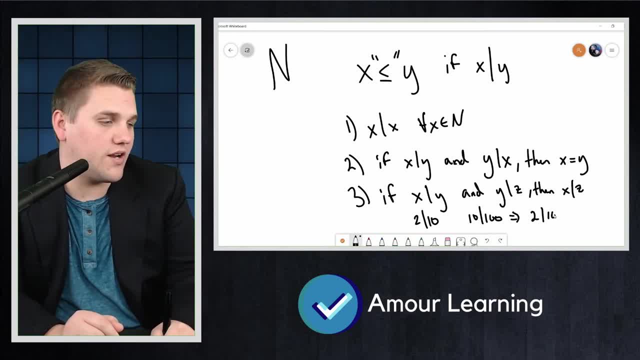 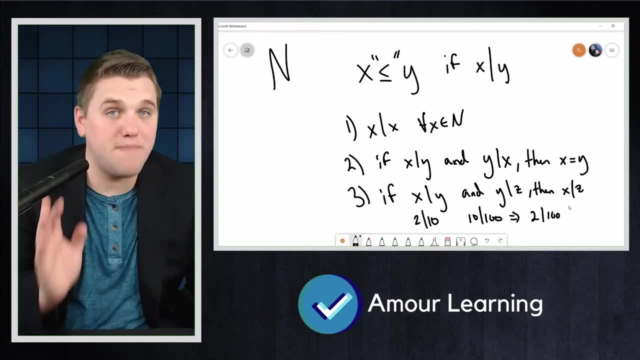 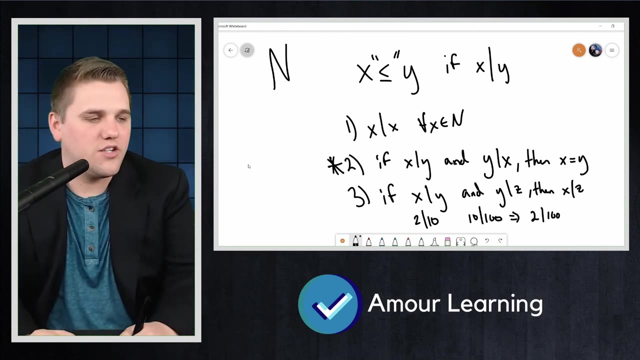 That literally means that 2 divides 100.. So notice that this relation is not symmetric, It's anti-symmetric. Again, this property, right here, is anti-symmetric And therefore it's not an equivalence relation, because x divides y does not necessarily mean that y divides x. So again the symmetric. 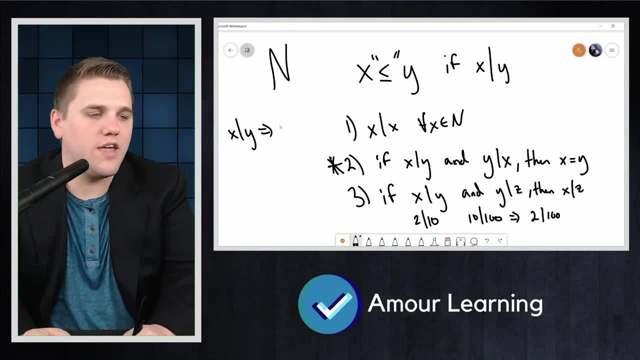 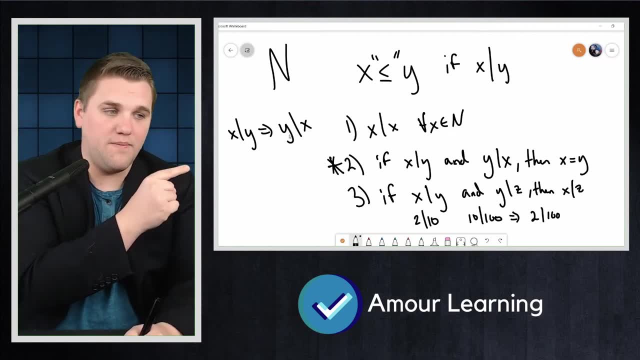 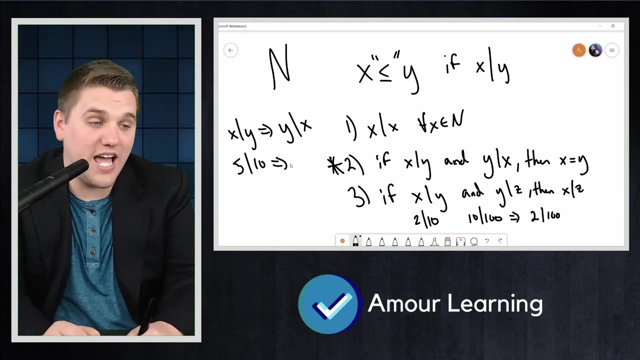 property was: if x divides y, then y divides x. If that were true, if this were true here, that would mean that the property divides or the relation divides is symmetric. But that's not true. That's not always true. For example, 5 divides 10 does not mean that 10 divides 5.. 10 does not divide 5.. 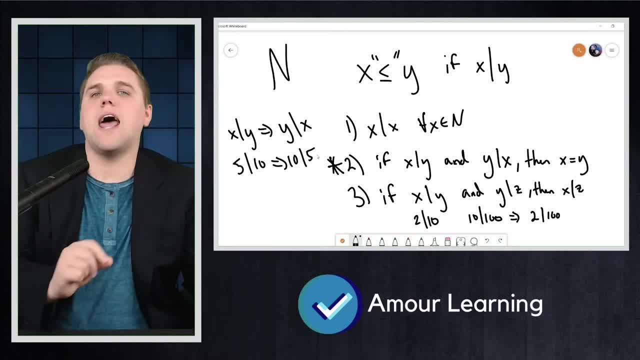 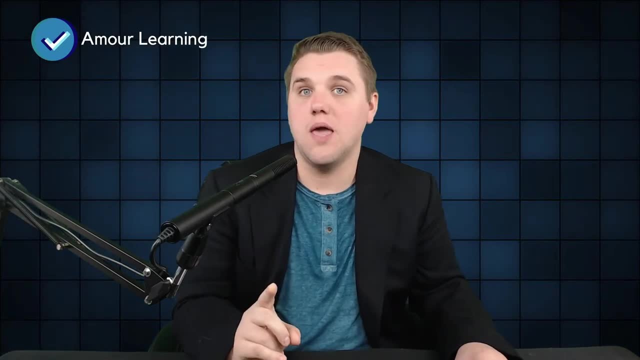 10 is not a factor of 5.. Now you might ask what is partial about partial orderings? Well, partial orderings don't have to be total orderings. A total ordering means that for any x and y in the 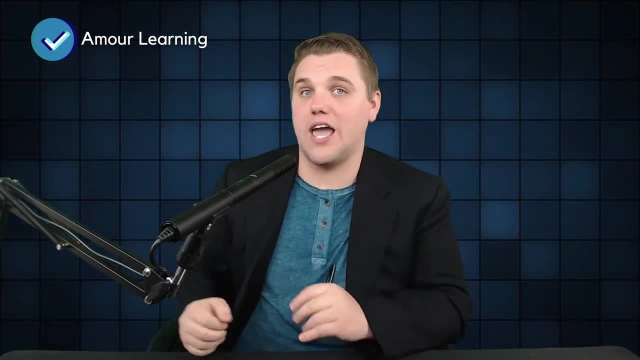 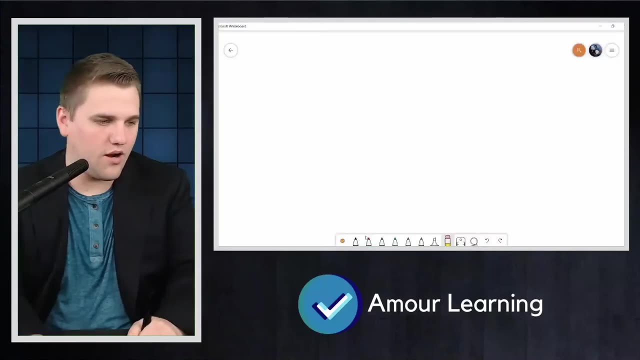 universe, either x is less than or equal to y, or y is less than or equal to x, And I'll write that out on the whiteboard here. So, in a total ordering, either x is less than or equal to y. 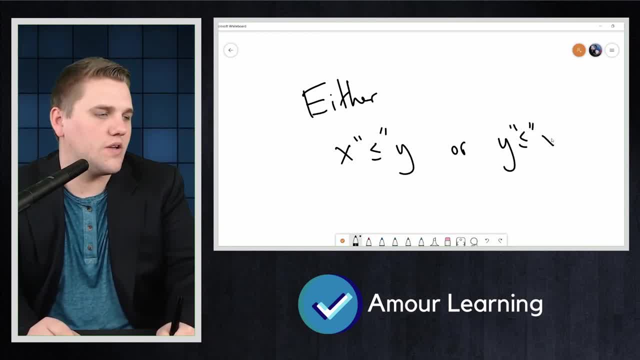 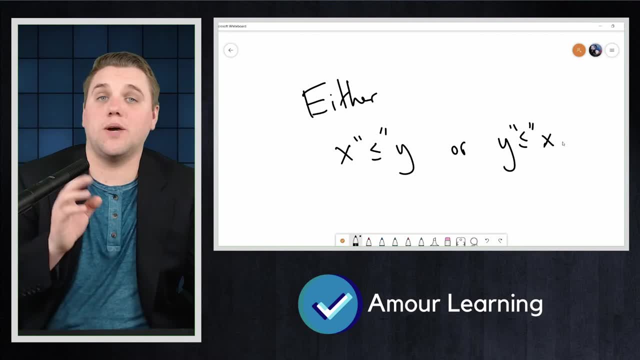 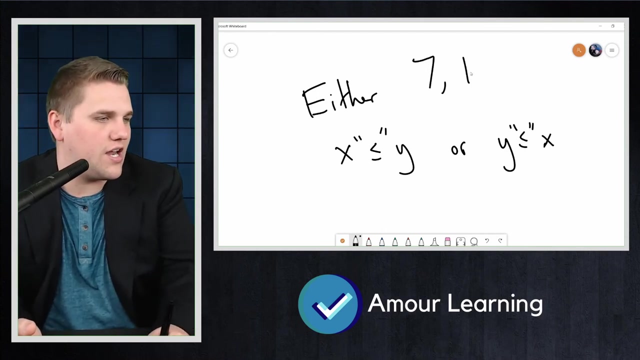 or y is less than or equal to x. So this means that x and y are comparable. Partial orderings do not necessarily have to fulfill this requirement. Take, for example, the divides partial ordering. If you take the elements 7 and 13,, then both 7 divides 13,. 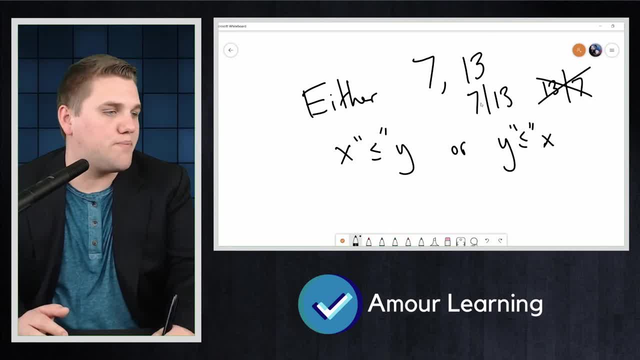 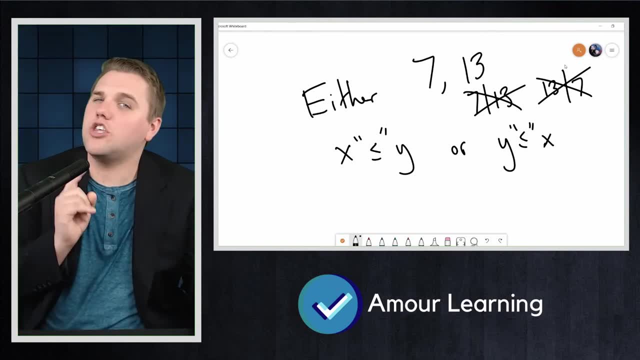 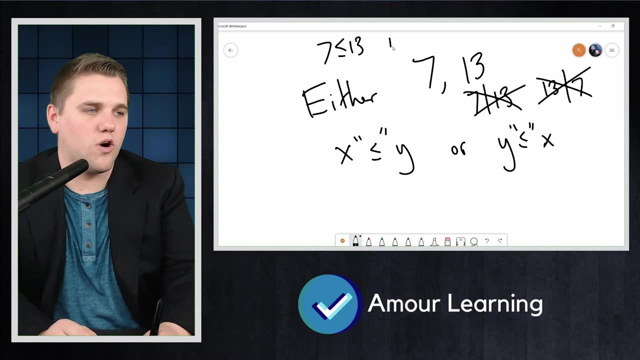 and 13 divides 7 are both false. These two elements are not comparable. Whereas under the usual partial ordering less than or equal to, we might say 7 is less than or equal to 13,, or 13 is less than or equal to 7.. One of those has to be true, and in fact. 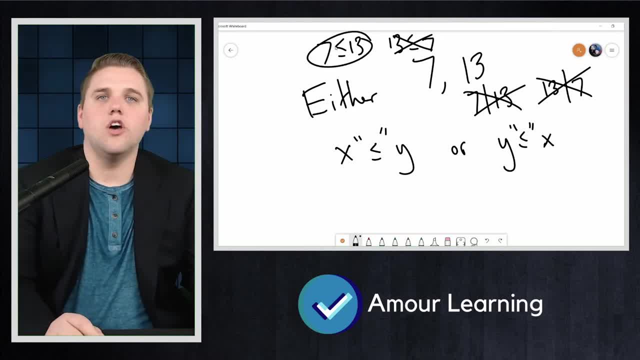 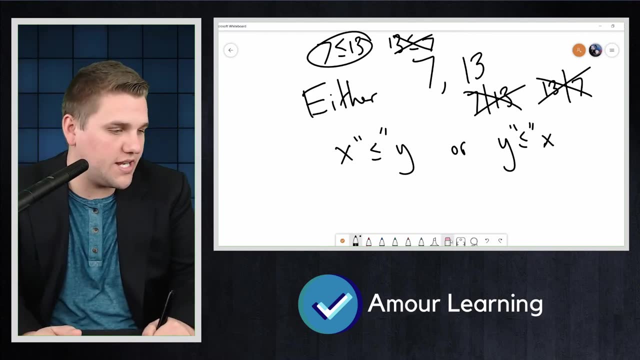 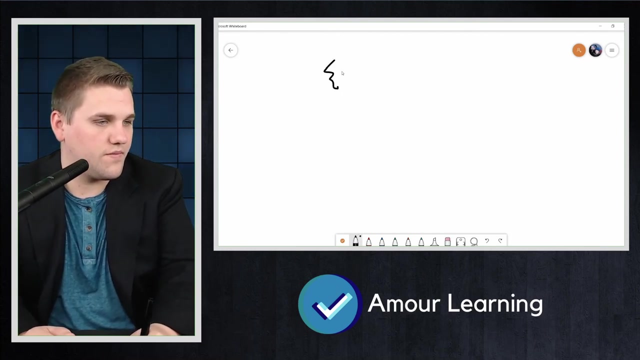 one of those. is true, that one specifically. Total orderings have many interesting properties. For example, they give rise to the concept of smallest and largest. For example, if I were to give you the subset 3, 8,, 5,, 10, 12.. 3, 8,, 5,, 10,, 12.. Yeah, 12.. What would you say is the least? 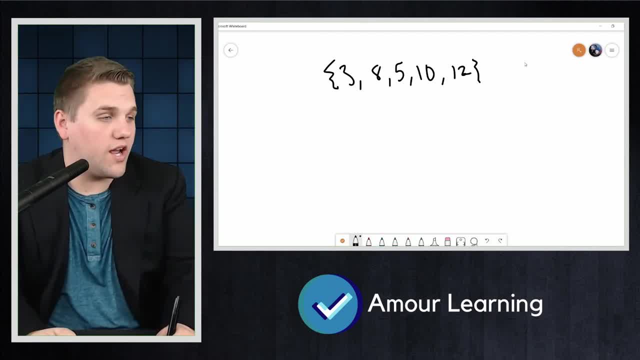 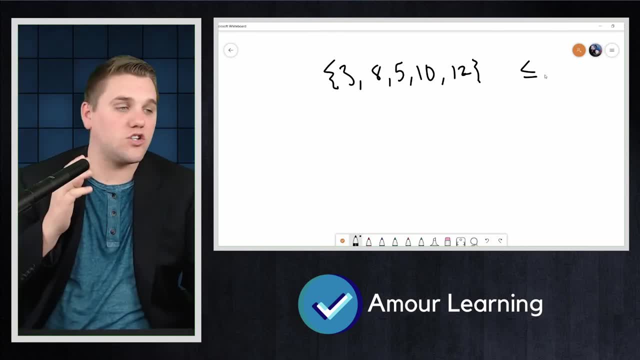 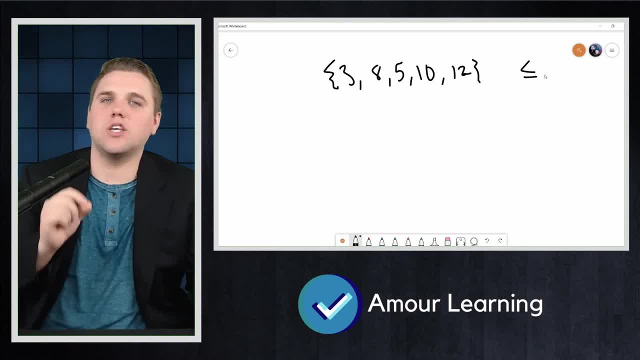 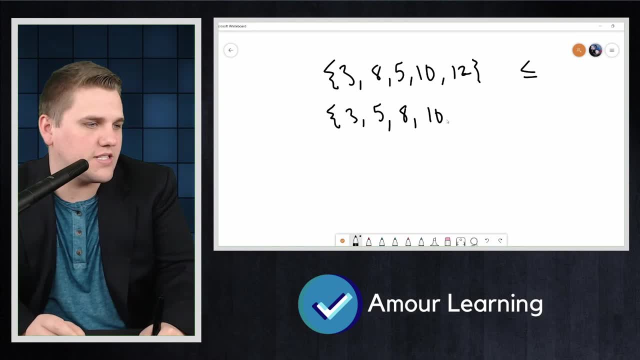 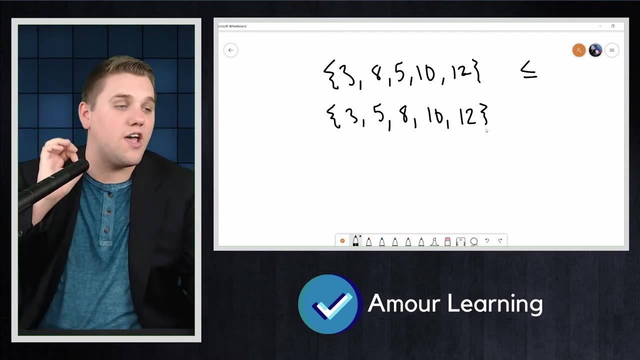 element. What you did is you took the set and ordered it as 3,, 5,, 8,, 10,, 12.. And then saw that this representation clearly shows that 3 is the least element. Well, under the usual ordering of. 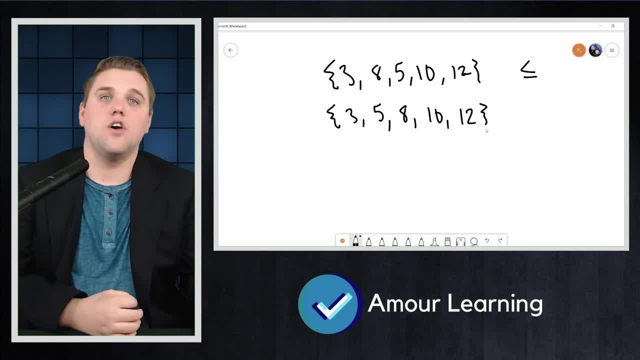 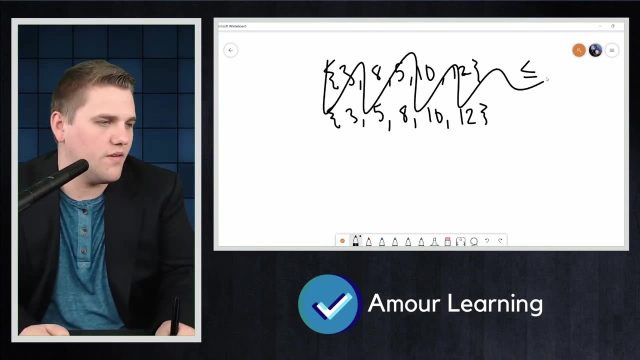 3 is the least and 12 is the greatest. With partial ordered sets that aren't totally ordered, there might not be a least element, For example, under the divides partial ordering. you might be able to say that if we're looking. 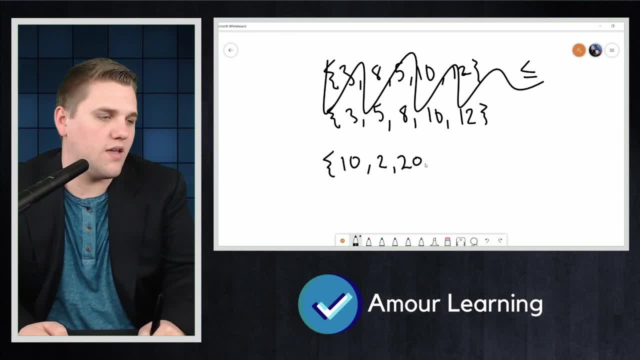 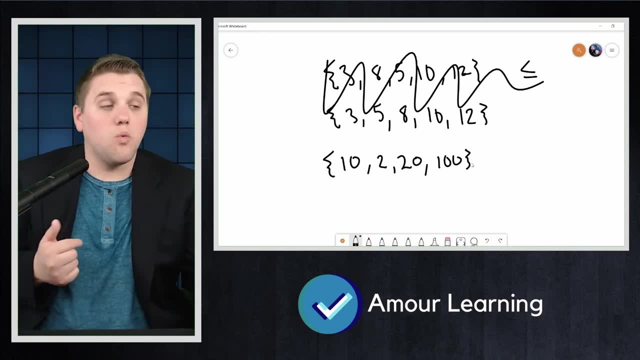 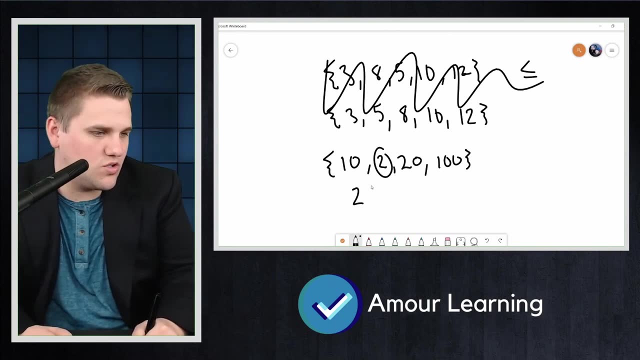 at the set 10,, 2,, 20,, 100,. what's the smallest element under the divides partial ordering? Well, this has a least element of 2, because we can order this as: 2 divides 10, divides 20, divides 100. 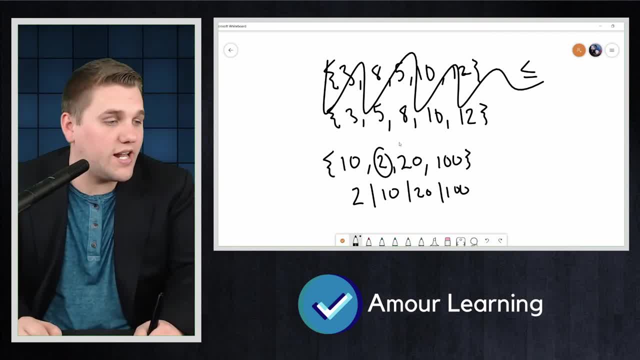 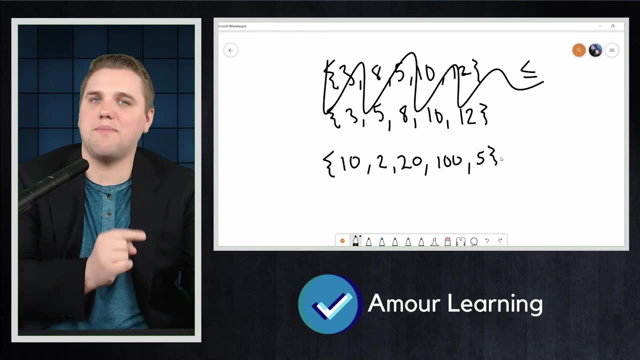 So this would mean that the least element is 2, and the greatest element is 100. But if we change this a little bit and throw in a 5 there, this will throw everything off. You can't be able to determine which is smallest, because 2 and 5 are not comparable under this. 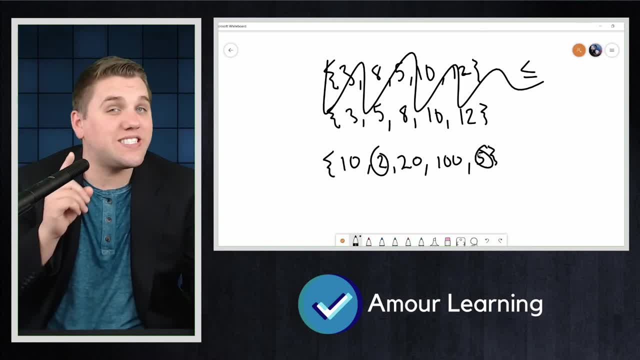 partial ordering of divides. You might be tempted to say that 2 is the least element, but that's because you are ordering. You are ordering the set under the WRONG relation. Under the divides, relation 2 and 5 are not even relatable whatsoever.